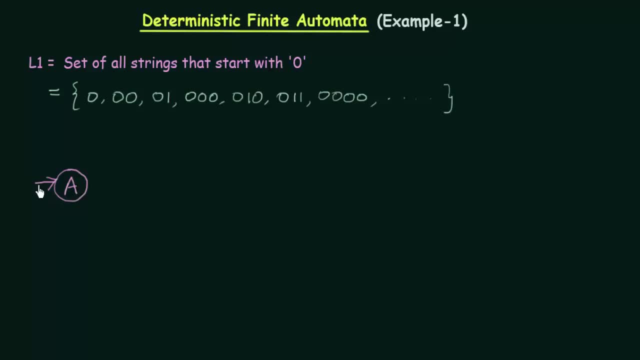 So I already told you in the previous lecture that whenever you see an arrow coming from nowhere pointing to a state, that shows that that is the starting state. So a is my starting state, So I am starting with a. Now, if I get input 0 in a, what will happen? 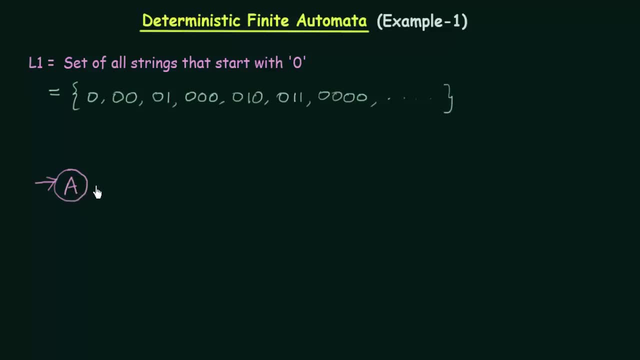 And if I get input 1 in a, what will happen? Let's see what should we do? Suppose I get input 0 in this a, I send it to another state which I call b Okay, and I put a double circle around this b. 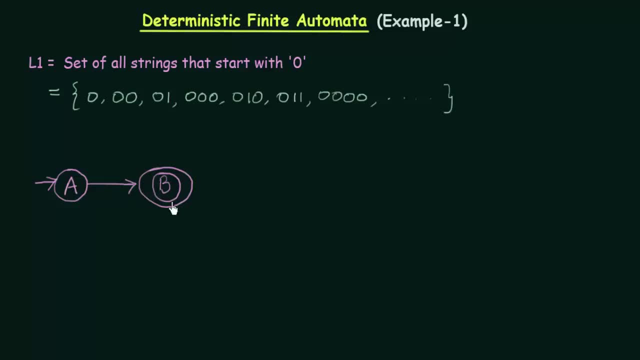 Now, what is the meaning of this double circle? Double circle means this is the final state. When you see a double circle, it always means that this is the final state. Now, when I give input 0 to a, it goes to b. 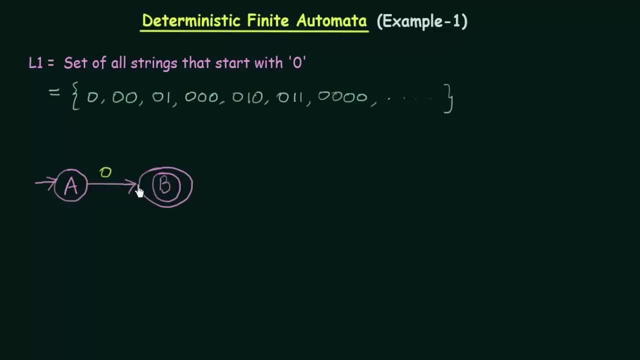 Now why is that? That is because I am to design a DFA that accepts all string that starts with 0. So a is my starting state and I am getting input 0. That means 0 is the first digit, And when 0 is the first digit, it goes to b, which is the final state. 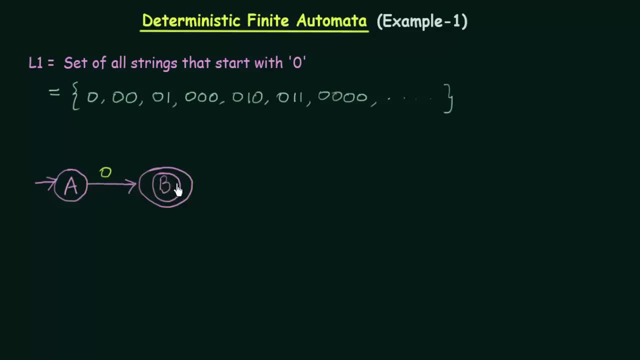 And whenever a string reaches the final state, that means that string is accepted, And whenever a string does not reach the final state, that means it is rejected. So whenever I am starting with 0, it should reach the final state because it should be accepted. 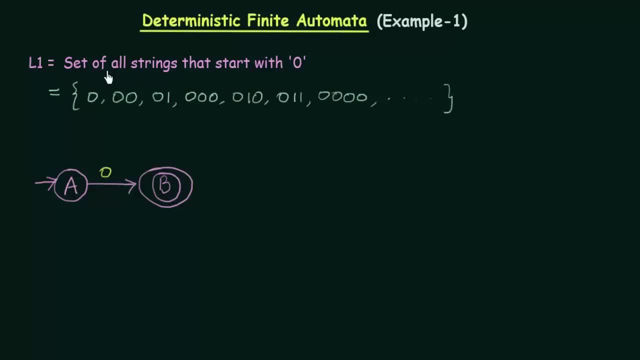 Why? Because I am to design a DFA for all strings that starts with 0.. Now I am in state b And after reaching state b, in b also, I can either get inputs 0 or 1.. So what will happen if I get either 0 or 1?? 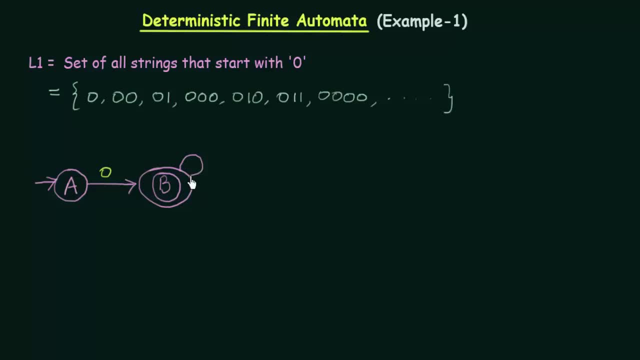 Since b is the final state, I will give a self loop here and I will write 0 or 1.. So what does this mean? This means that after reaching this final state b, whatever input you get after that- whether it is 0 or 1, it stays in the final state b itself. 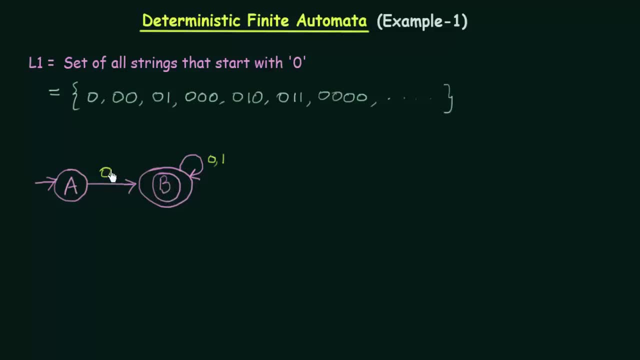 Okay, Because the string started from 0 and our only condition is that it should start with 0. So it starts with 0 and after it reaches the final state, whether it is 0 or 1, it doesn't matter, It stays in the final state and that string will be accepted. 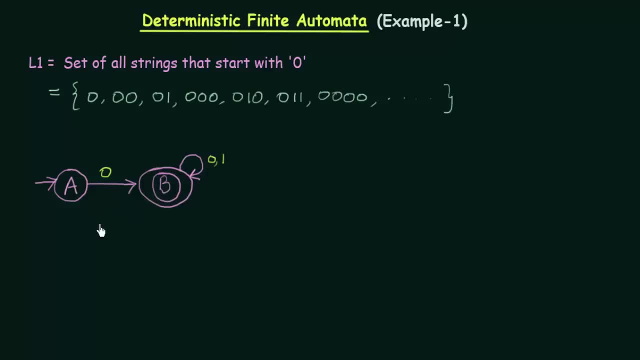 Okay, I hope that was clear. And now is this complete? No, This DFA is not complete. Why? Because we already mentioned what will happen if a gets the input 0. But we did not mention what will happen if a gets the input 1.. 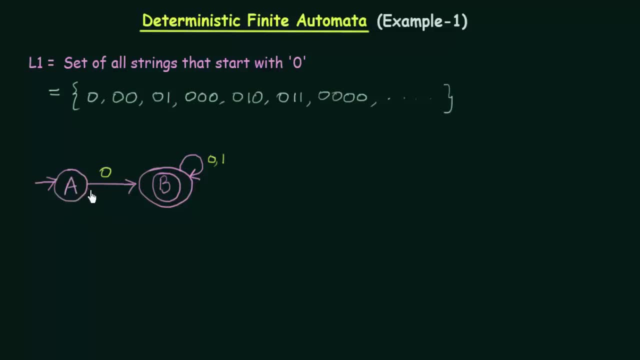 So a is my starting state, and if I get input 1, that means 1 is the first digit. And should that be accepted or not? No, It should not be accepted. I should accept only those strings which start with 0.. 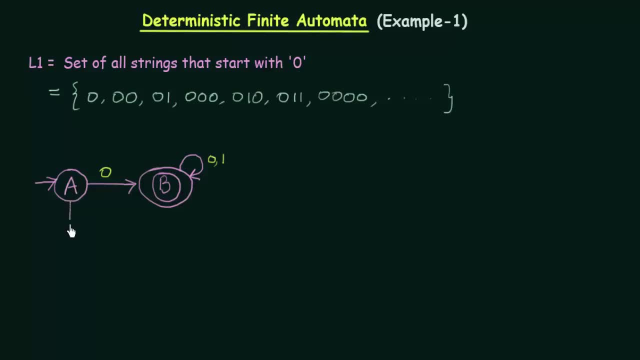 So if it starts with 1,, what will happen? I will send it to another state, which I call state C. Okay, I send it to another state called state C When the input is 1.. When the input is 1, it goes to state C. 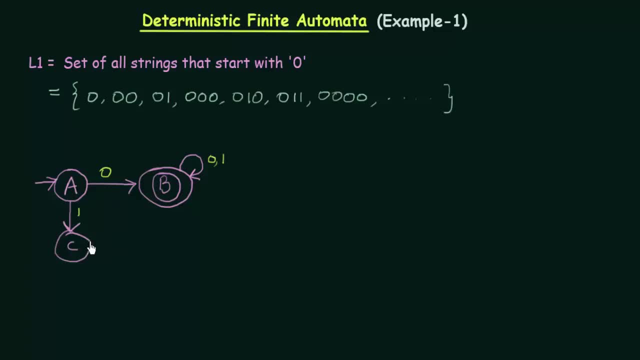 And in state C. after reaching state C, whatever input I get in state C, it stays in state C itself, Whether it is 0 or 1.. Okay, So if a string starts with 1, this is my starting state. 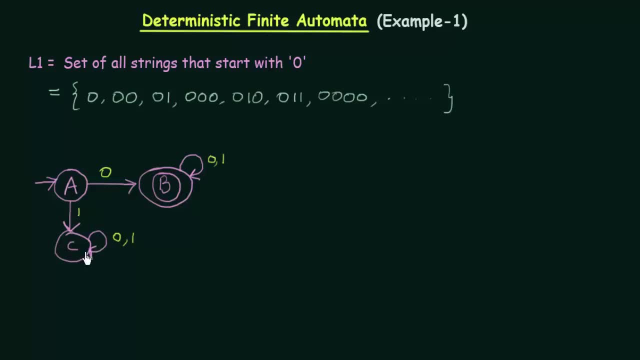 If it starts with 1, it goes to state C And after reaching state C, whether it is 0 or 1, it stays in state C itself And it cannot go back to this final state anymore. Okay, It cannot go to this final state anymore. 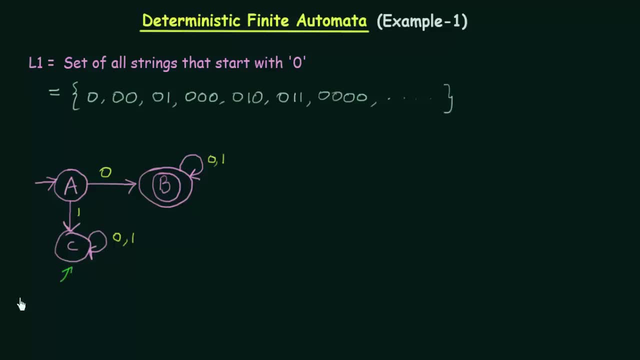 So this kind of state is known as dead state, Dead state, or it is also known as trapped state, Trapped state. Why is it known as dead state or trapped state? Because once you reach here, it is trapped over here. It cannot reach the final state anymore, which is B. 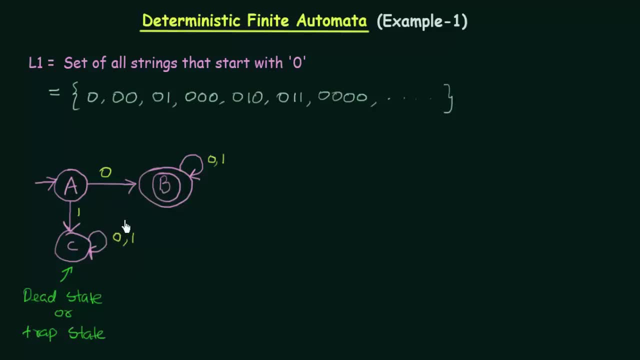 Okay, And when a string cannot reach its final state, that string will be rejected. Okay. So now my DFA is complete, Because I have already mentioned in A, if I get 0, it goes to B, If it gets 1, it goes to C. 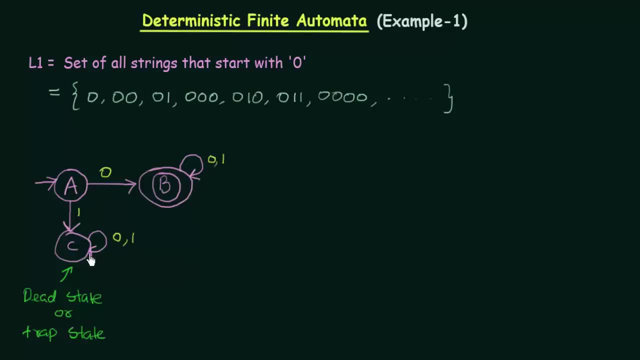 It is complete. And in B, whether it is 0 or 1, it stays in B itself. And in C, whether it is 0 or 1, it stays in C itself. Now my DFA is complete. Now I have designed the DFA for the set of all strings that starts with 0. 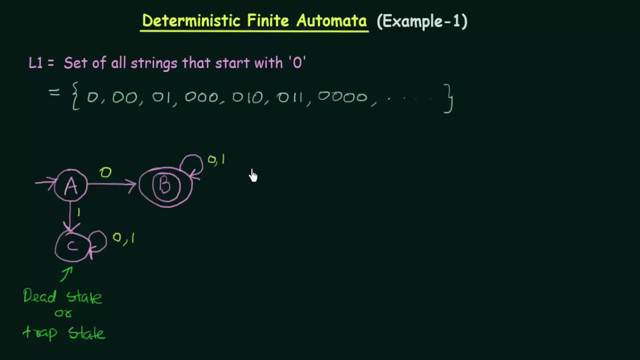 Okay, Now let us check if this is correct. Let us take a few examples to see if this is working. So in my first example- let me take an example- I want to check the string 001.. Okay, So I am going to check for string 001.. 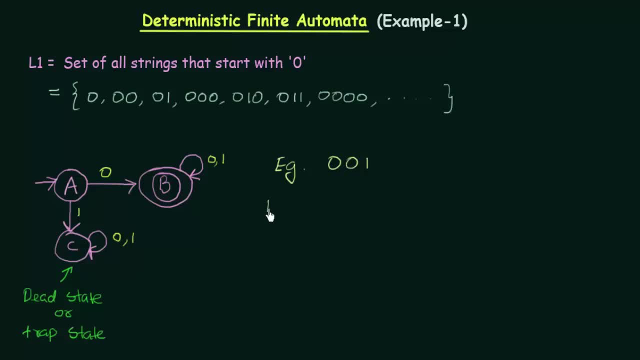 So it always starts from my initial state, My initial state, Initial state, which is A. I start from state A Right, Because A is my initial state And I get input. I give input 0.. On getting input 0, what happens? 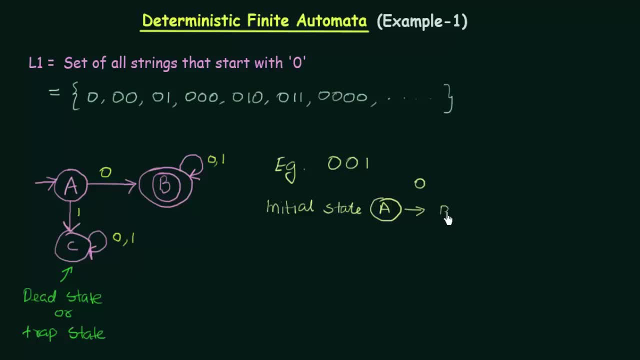 A goes to B, A goes to B And the next input is 0 again. So I am right now in state B, Right, And if I get input 0, what happens? B, it stays in B itself. It stays in B itself. 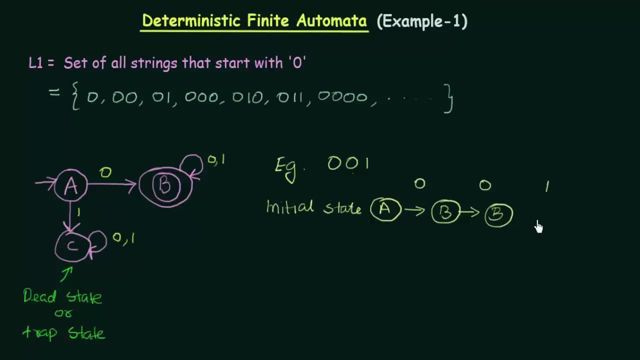 And then the next one is: the next input is 1.. So what will happen? I am in state B, And if I get input 1, what happens? It still stays in state B, Right, And here I reach the end of the string. 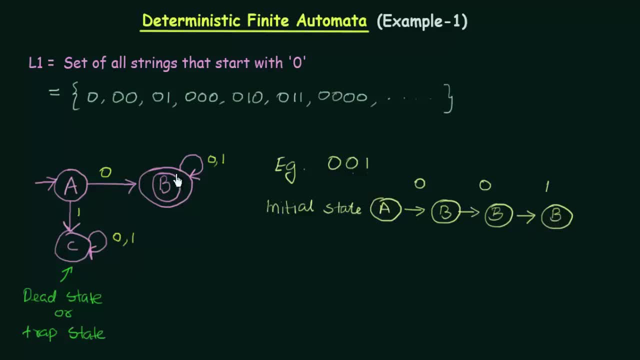 And at the end of the string, what is my position? I am in B, I am in B And B is it the final state? Yes, it is the final state. B is the final state, Right? So since B is the final state, this string should be accepted. 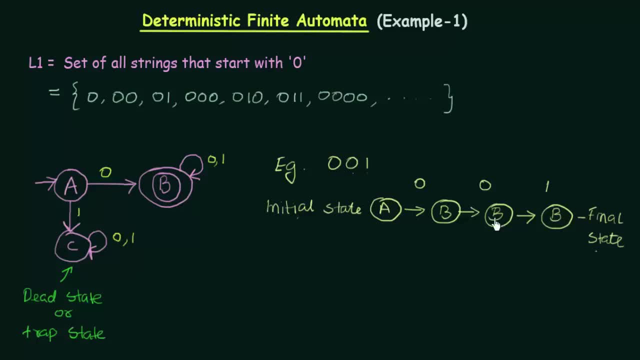 Why It could start from the initial state and it reached the final state. Since it could reach the final state, this is accepted. Alright. Now let's take another example. Example number 2 is 1, 0, 1.. 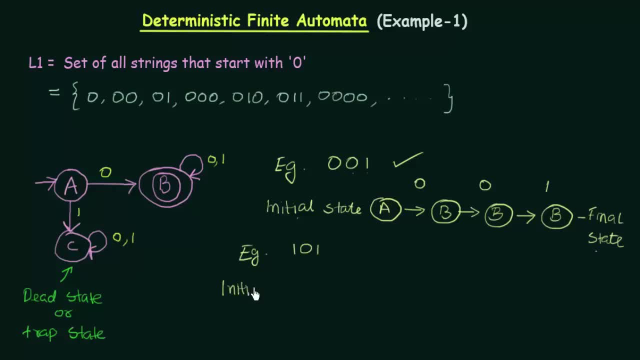 Again, I start from my initial state. What is my initial state? It is A And I get the input 1.. 1 is the first input And on getting input 1, where does A go? It goes to state C.